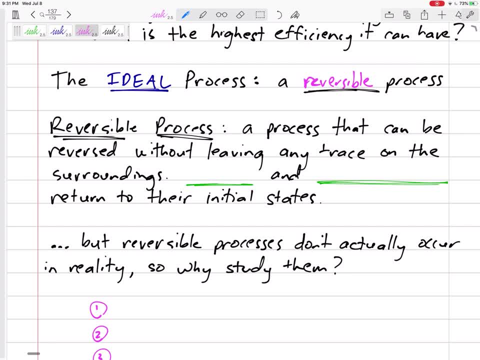 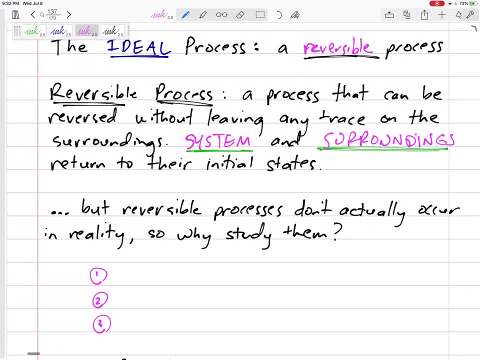 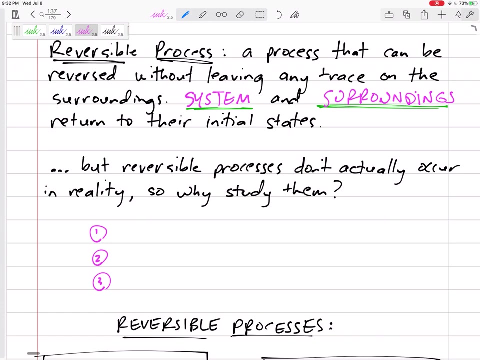 A reversible process is a process that can be reversed without leaving any trace on the surroundings, So both the system and the surroundings have to return to their initial states. Reversible processes don't actually occur, right. They're theoretical. Why would we study them? A few reasons. 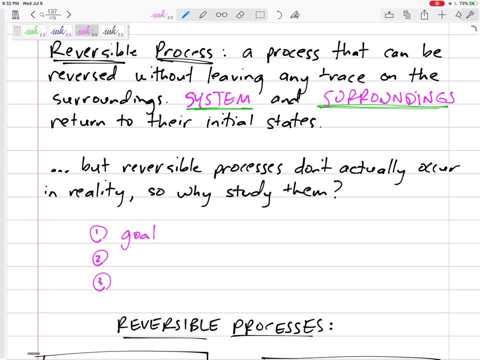 Because that's kind of our, That's our goal, That's what we're aiming towards. We're seeing who can get the closest. We don't know if nobody's going to get there, but who can get there and how close to them can we get? 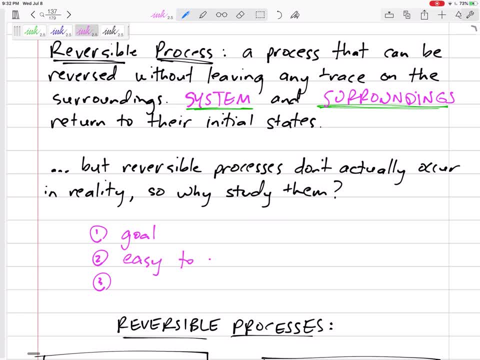 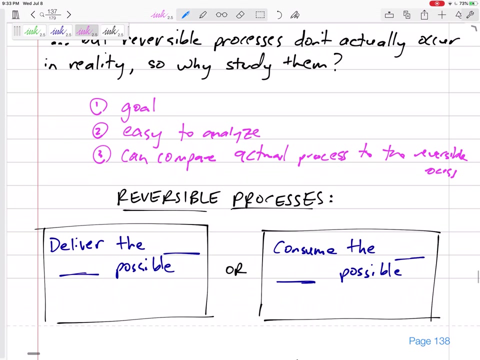 Also. one reason is they're easy to analyze. Alright, sometimes the math, the equations are easier for reversible processes, And so what we can do is we can compare Our actual process to the reversible process. Okay, reversible processes are the ones that will deliver the most work possible. 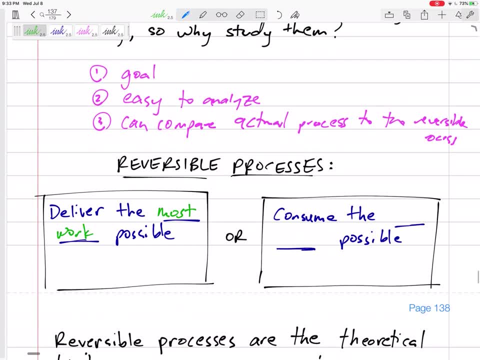 if that's what we're aiming for, right. If, like a car engine, right Car engines, We're trying to get work out, We're trying to get work out of it. A turbine, We're trying to get work out of it. 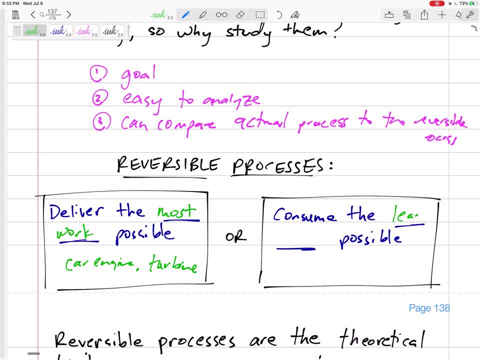 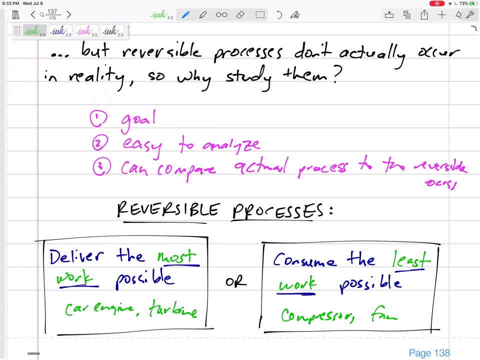 Or the flip side of that may be. what we're really trying to do is trying to use something that will consume the least amount of work in, like a compressor Fans. So it depends on what type of a process it is, But reversible processes are the ones that are the best, the ideal. 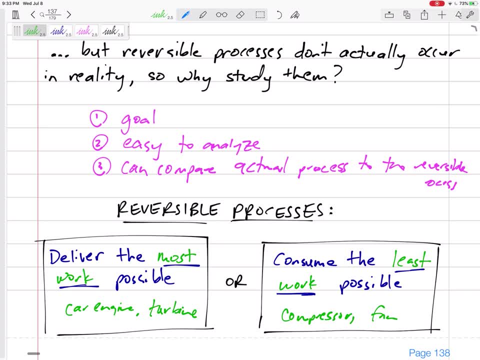 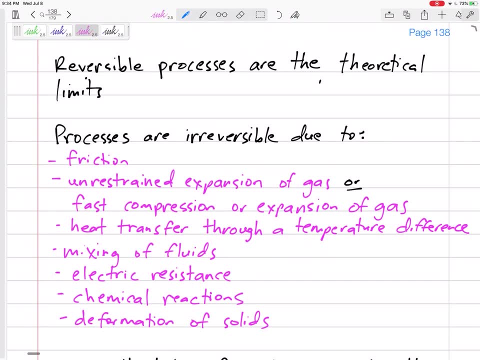 They'll give you the most work if that's what you're wanting, or they'll consume the least work if it's that type of process. Reversible processes are the theoretical limits. I like to call it the unreachable. Unreachable goal, Alright. 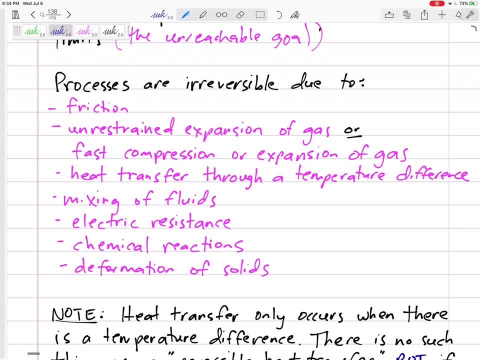 We're not going to have reversible processes In nature, in real life, because of friction, because of unrestrained expansion of gases or fast compression or expansion of gases, heat transfer through temperature differences- All of these make processes irreversible. Mixing of fluids could be irreversible. 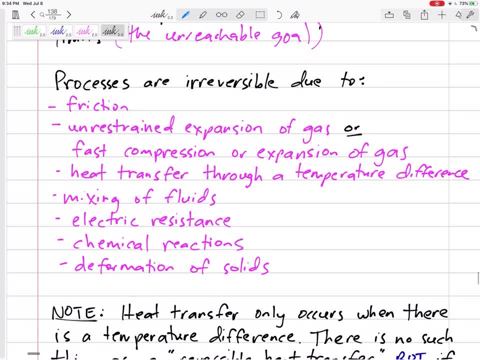 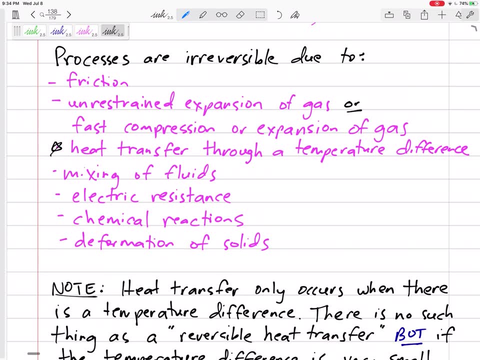 Electric resistance, chemical reactions, deformations of solids- these are all irreversible, So we're going to have a little bit of some of these Right here. Heat transfer through a temperature difference. The only way we have a heat transfer is through a temperature difference. 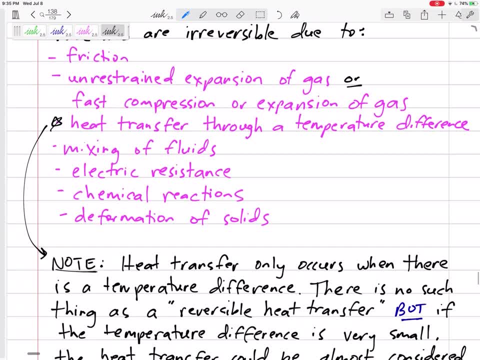 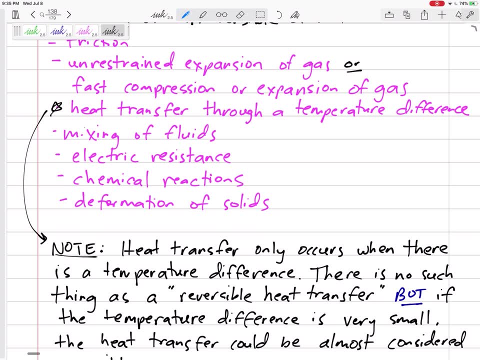 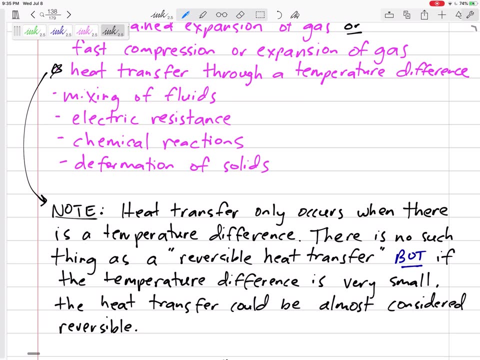 So that's why there's Processes are never going to be reversible. Alright, so heat transfer only occurs when there is a temperature difference. There's no such thing as a reversible heat transfer, But if we can get the temperature difference as small as can be. 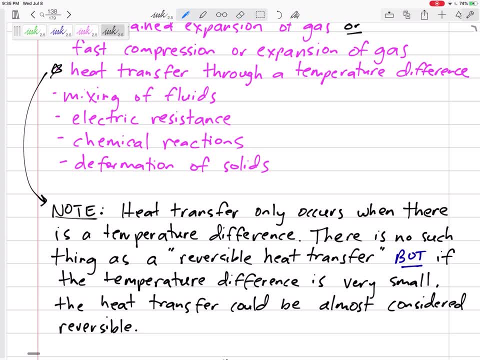 then we can always- Almost, you know, consider it irreversible. So we're going to have some heat transfer through temperatures that are the same temperature. Okay, That's a reversible heat transfer. if that makes sense, We're going to assume those temperatures are as close to the same. 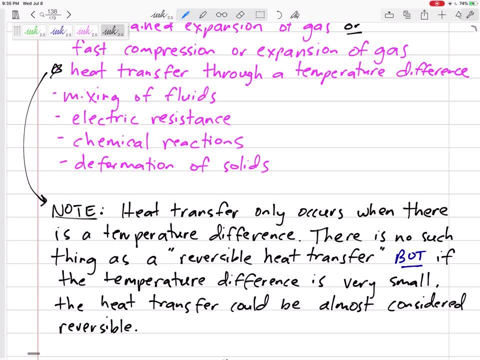 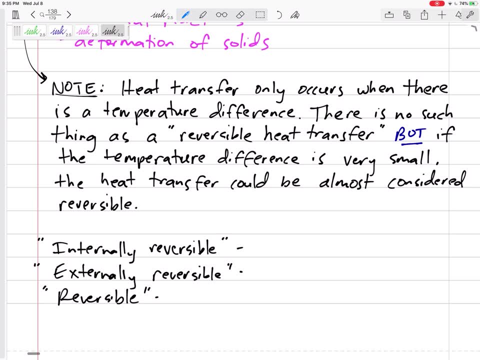 There's a very small temperature difference, So that it's almost reversible, Alright. Alright, some things could be internally reversible Reversible, or externally reversible, or actually reversible. Internally reversible is reversible inside the boundaries, So this is the system, right. 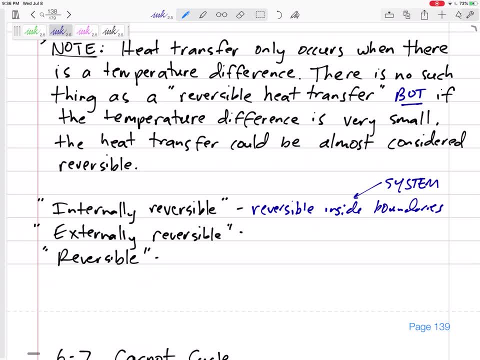 Our object is reversible. Externally reversible is reversible outside The boundaries, Right, The surroundings. But in order for something to be reversible, actually reversible, then both the system and the surroundings have to be reversible, Both internally and externally reversible.